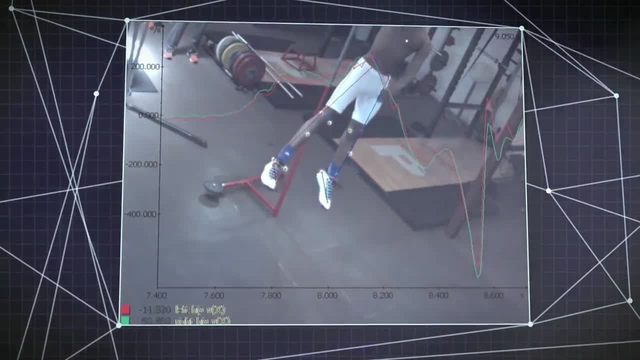 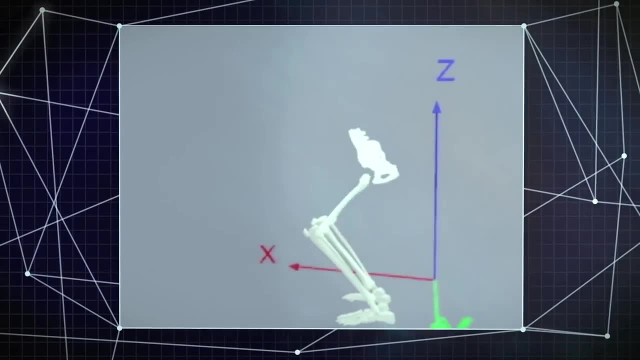 at peak forces. when athletes land, Nobody talks to them about how your foot should interact with the ground. but it turns out two athletes coming down from the same height can completely change how forces are transmitted through their bodies. If these systems we're assessing don't have correlations, 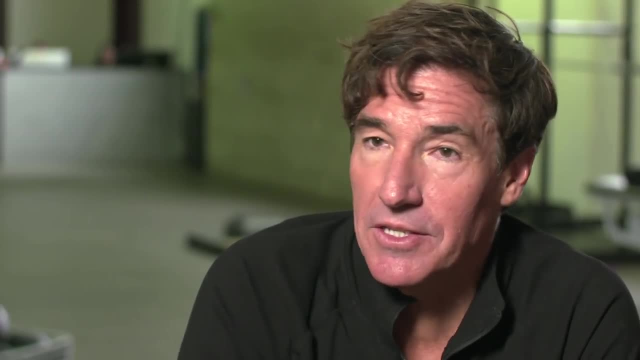 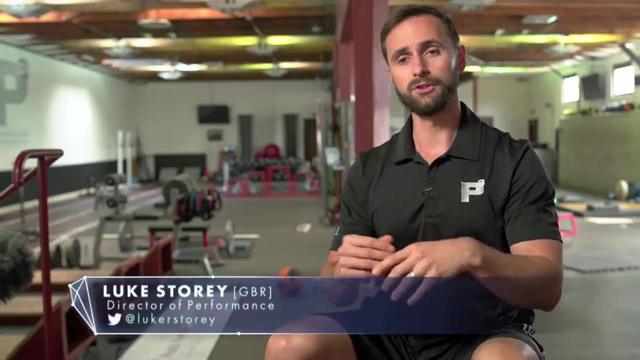 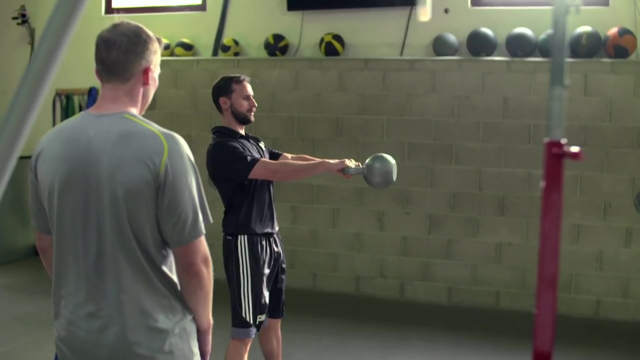 on court, on field, then there's no reason to do this assessment. We try to make our programs as individualized as possible And that comes from using our sort of our technology, whether that be force plates or 3d motion capture. We can compare it to positional peers or 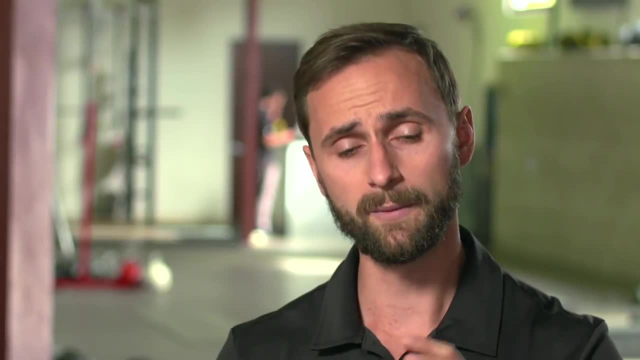 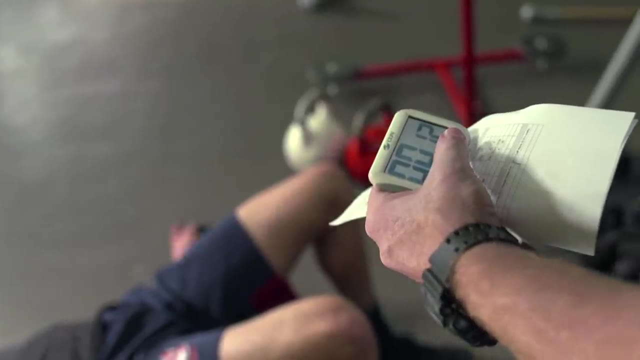 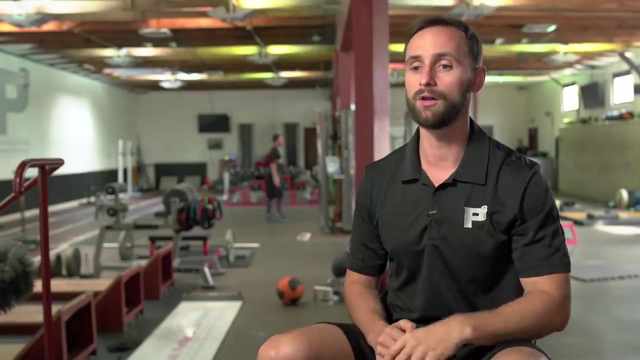 athletes in their age category, whatever it may be, But ultimately there will still be some subjective viewpoints of how we actually write the program. We also use our technologies to look at sort of the athletes fatigue and the athletes sort of current acute physical state where they're at as well. so we can 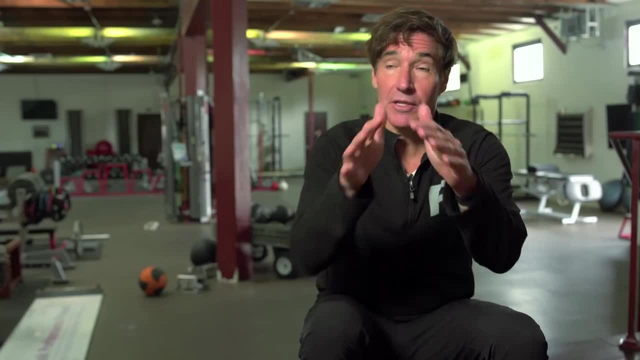 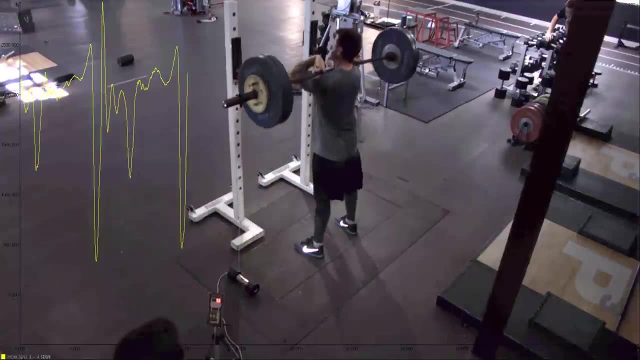 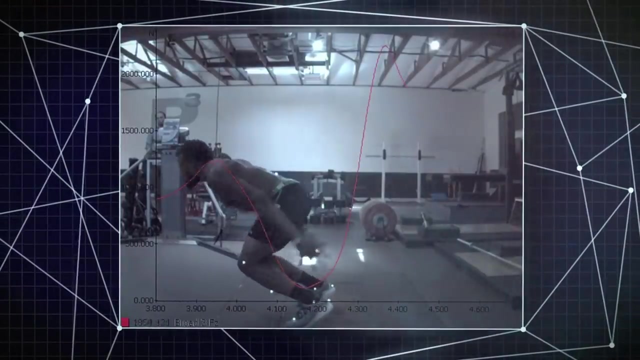 change the program accordingly. It's very difficult to bring those two pieces together To take this data, understand the highest yield pieces of that data and then use it to generate actionable prescriptive models. You need a confidence on both sides, on the objective data development and technology side, as well as the pure training athlete. 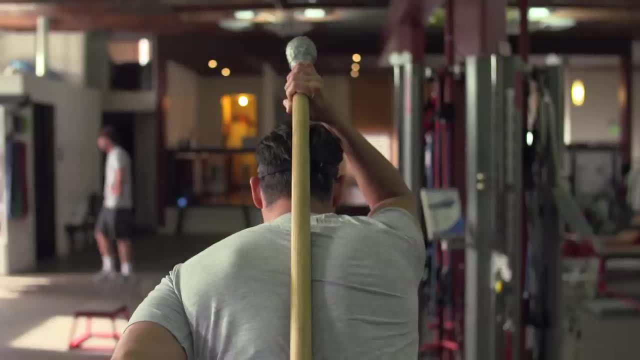 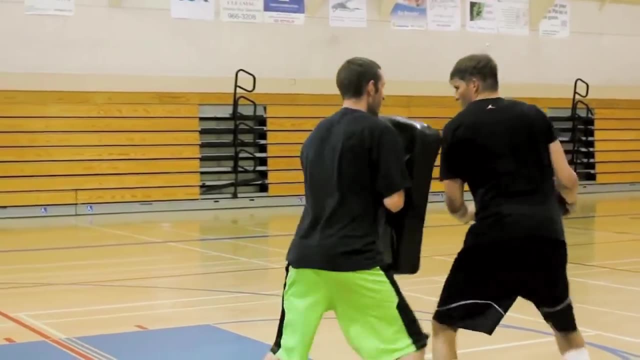 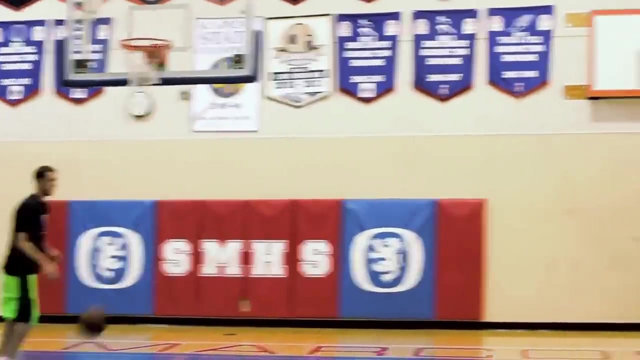 development side. I think that the biggest challenge early on was the fact that there wasn't a sports science infrastructure. Teams, strength coaches- they're not used to having these granular perspectives on their athletes. They just want them working hard As long as they're working up a sweat. 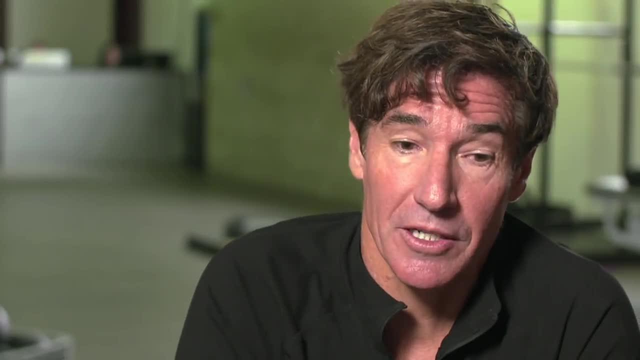 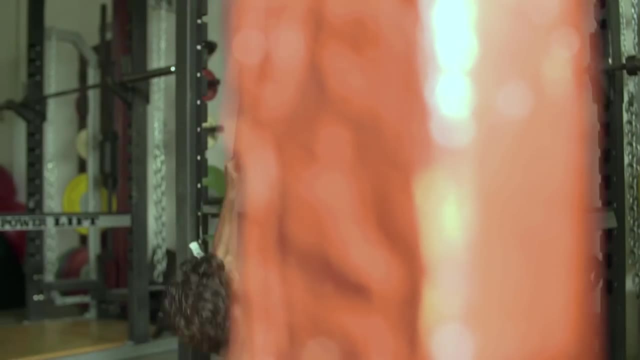 you know things are good. The athletes still need to sweat, They need to work hard, But if we can do this really, really smartly, then we're gonna optimize careers, There's no doubt about it. Every injury that an athlete develops, other than the big traumatic injuries, they telegraph themselves in subtle ways, or 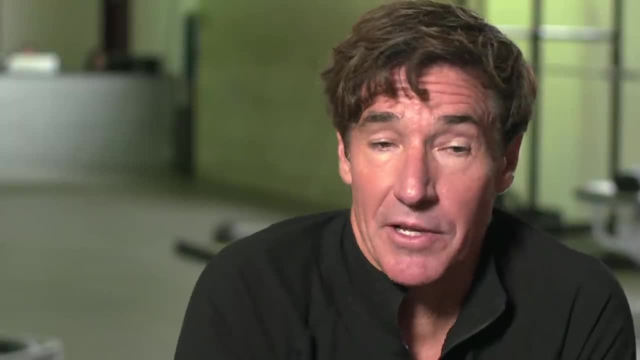 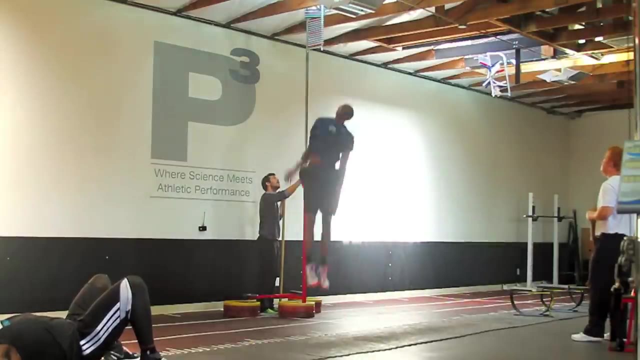 not such subtle ways. There's a reason that a 25 year old NBA player has no cartilage on the medial aspect of his body, On the medial aspect of his left knee. It didn't come out of nowhere, But up until now there wasn't a real 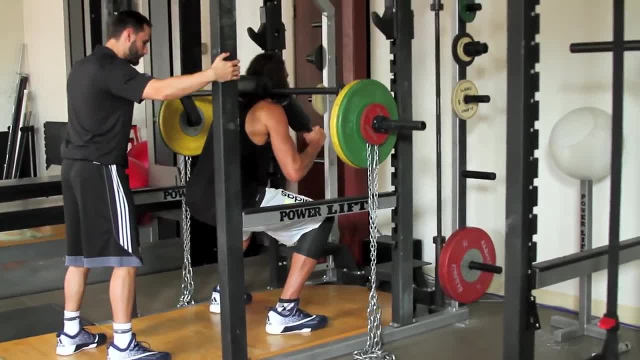 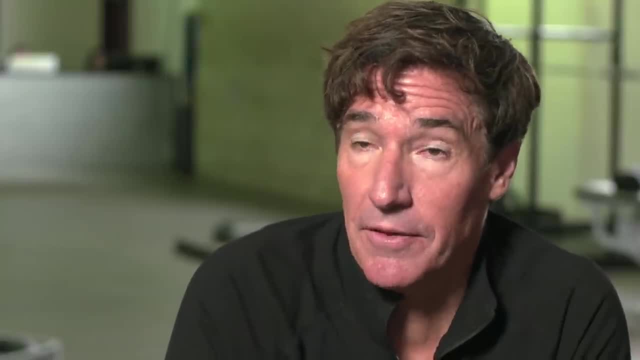 vigilant effort to understand those signals before that injury was developed. Generally what happens is an athlete just plays until he can't play anymore and the thing hurts too much and then it gets worked up. You go see an orthopedist, you get images and you find out what's going on with it structurally. 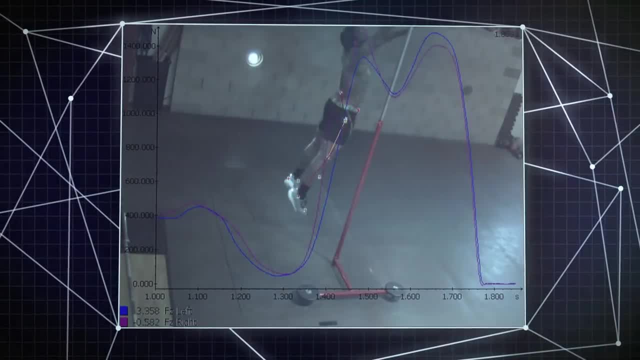 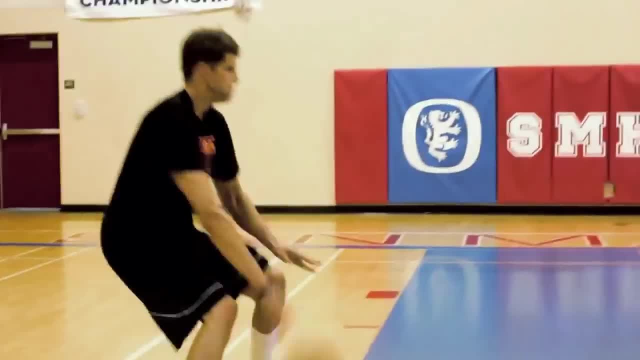 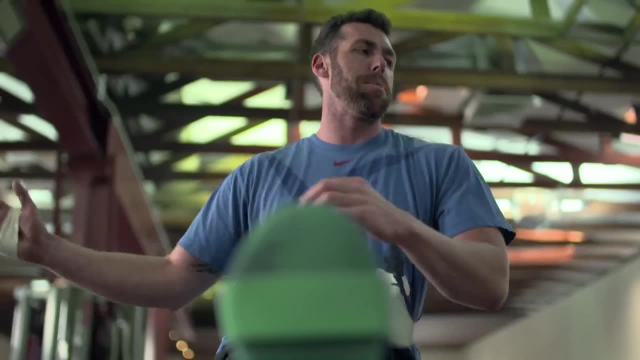 the data to be able to ask those questions. When you have athletes that will come back year after year, you can really start to see exactly those changes over time. So someone like Dylan Axelrod will be here for four months. We can assess him three to four times during that time and we can really change the program. 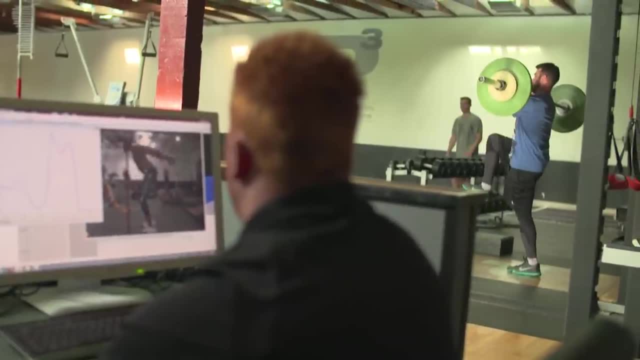 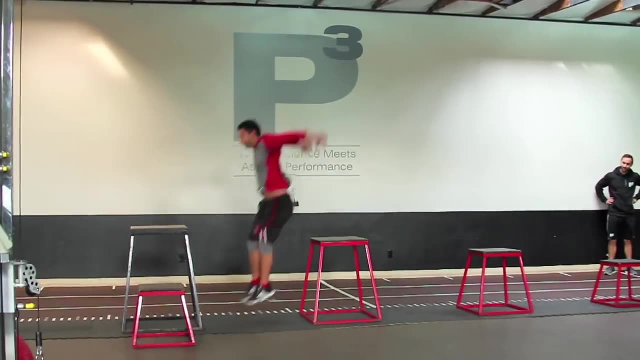 accordingly, It's our responsibility to make the athletes life better with the data we collected, and that means being smarter about how we train them. It means not doing something we would have done if we didn't have this insight into how he works, And it means using this data to enhance his career as he goes forward. 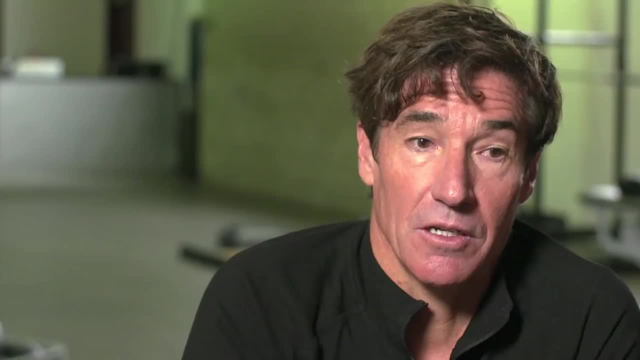 You know we're working in this space with the subjective assessment of athletes and all the data we have on athletes. that hasn't existed before. What we're doing is damn fun and exciting. 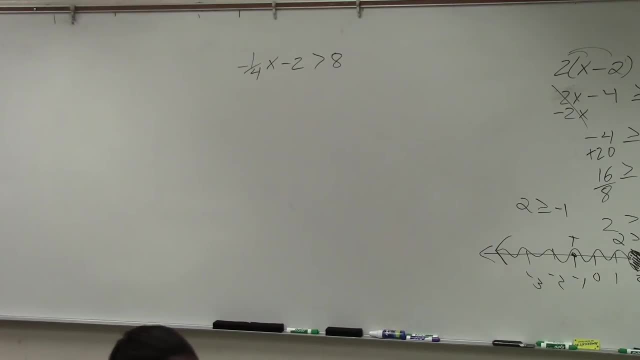 OK, So on this case we have negative 1. fourth x minus 2 is greater than 8.. Now I had a lot of problems with students because right now your hour is up. just saying You guys, now we're running out of your time. 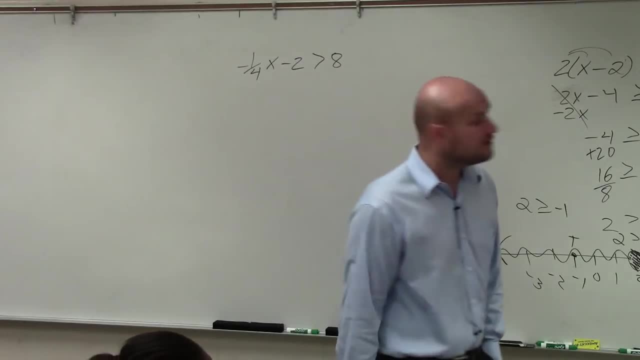 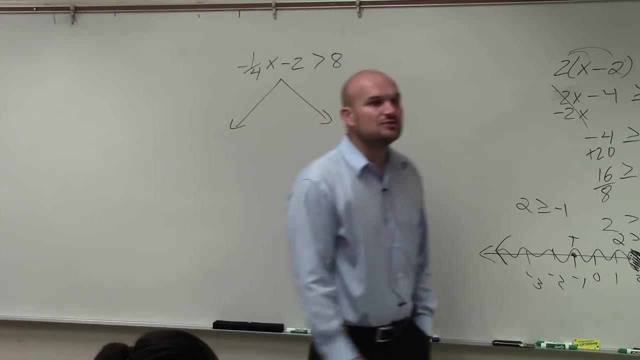 There's two different ways to deal with this, And we've been going over this over and over and over again for fractions. So there's two separate ways to do this. The first way, ladies and gentlemen, is to get rid of the fraction. 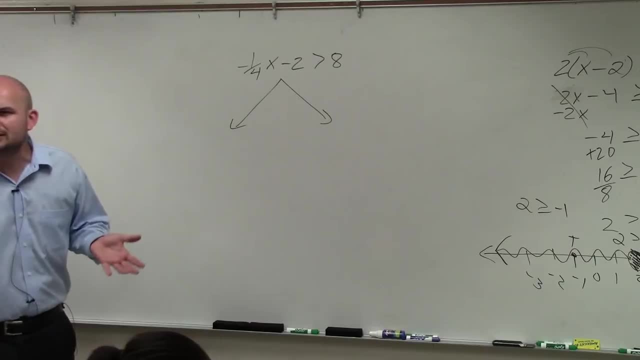 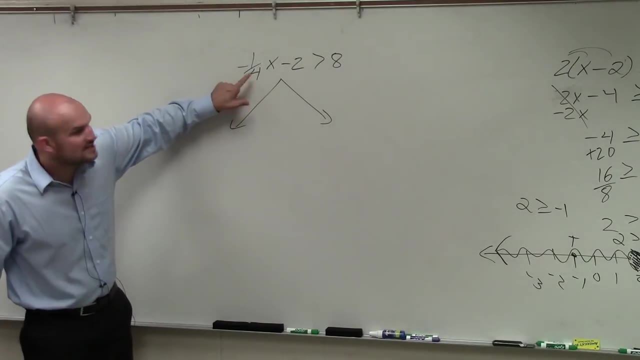 Why do we have a fraction here? The reason why we have a fraction? the reason why we have a fraction is because 4 does not evenly divide into 1.. Or you could say negative 1.. Doesn't really matter what you think of the negative.